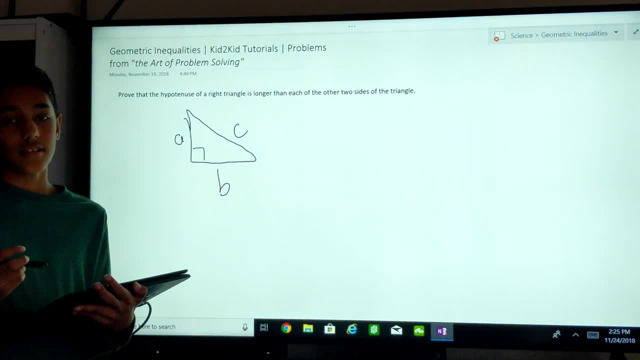 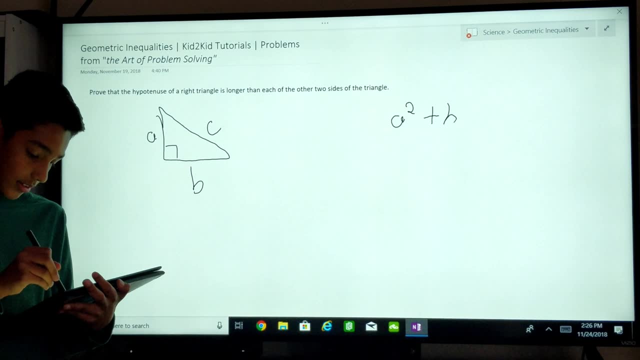 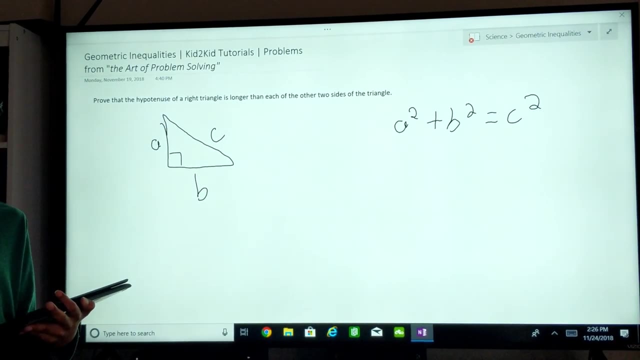 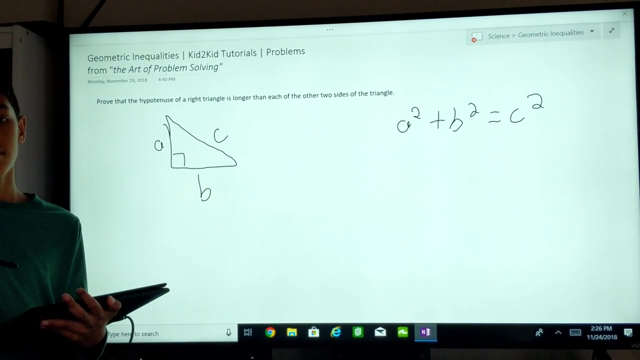 Since this is a right triangle, we can use the Pythagorean theorem. so let's put it out here: a squared plus b squared equals C squared. So we know that C squared has to be greater than A squared. This is because if A squared was equal to or larger than C squared, then this wouldn't 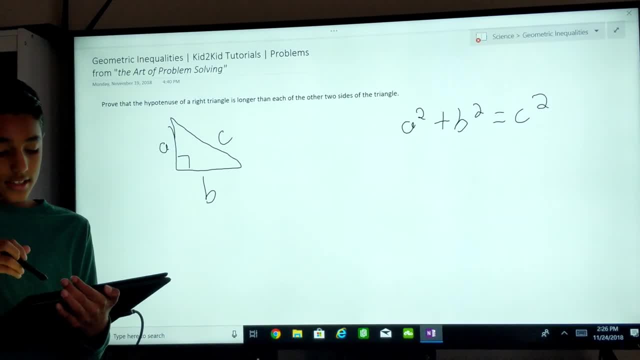 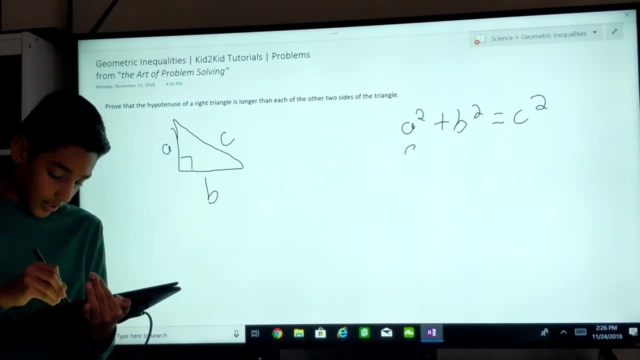 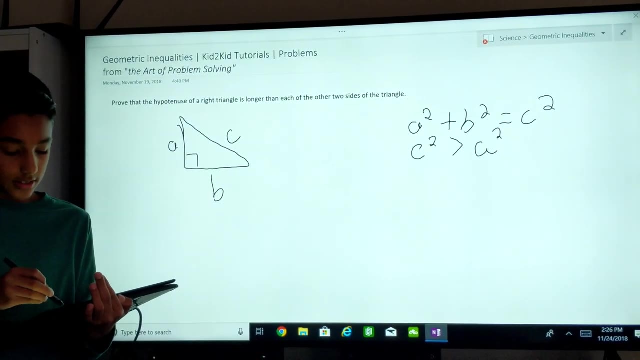 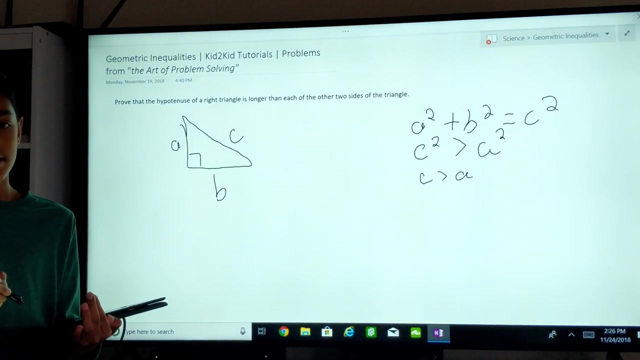 be equal to C squared, to c squared, because you have to do that plus b squared. so it wouldn't make sense if a squared was larger than c squared. so then we know that c squared is greater than a squared, so we can take the square root of both sides and we get c is greater than a. so the same thing applies to. 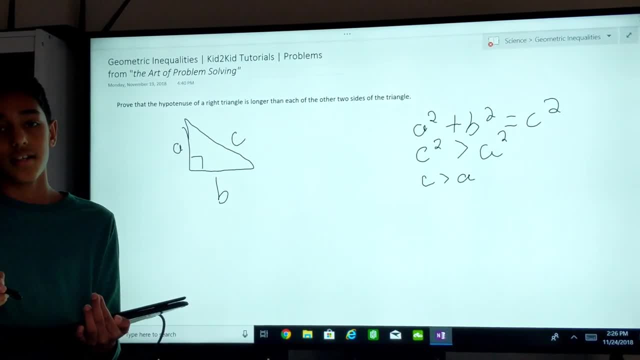 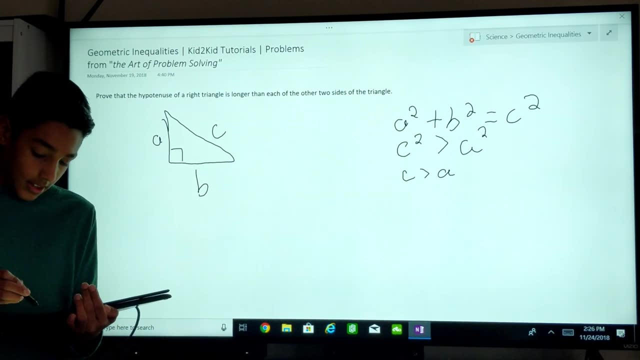 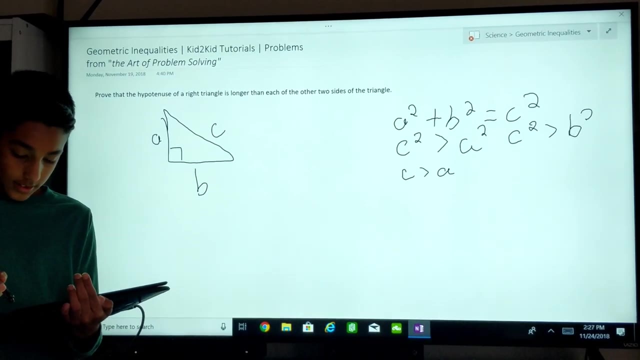 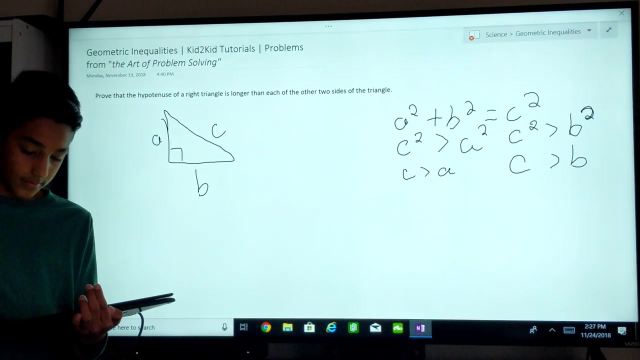 c. if b squared was larger than squeeze c squared, then that wouldn't make sense, because we still have to add a squared to b squared and that would have to equal c squared. so c squared is also greater than b squirt. so that means c is greater than b. so now let's go back to the basic equation. 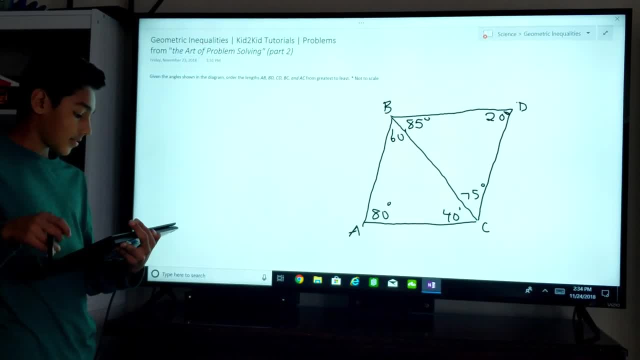 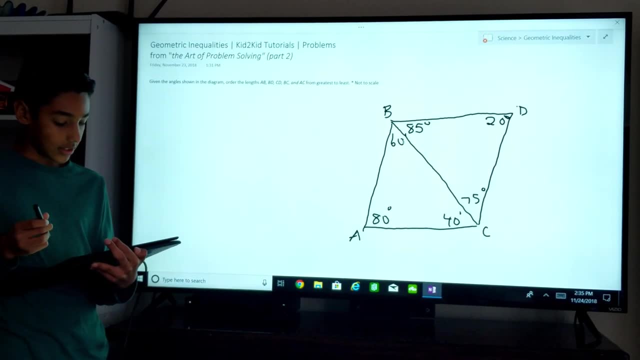 and apply for the product of plus c squared. so let's work on the model we have the product of. to our second and final problem. so this one says: given the angle shown in the diagram, order the lengths a, b, b, d, c, d, b, c and a c from greatest to least. so this figure is not drawn to scale. 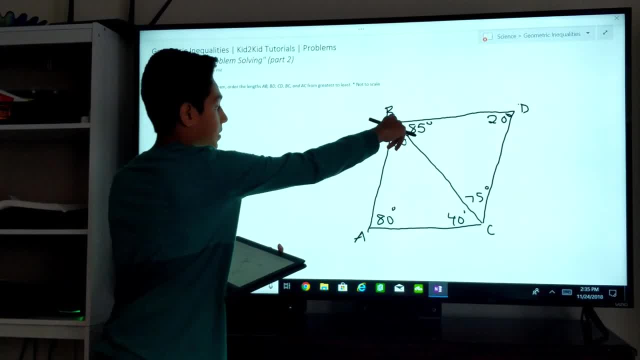 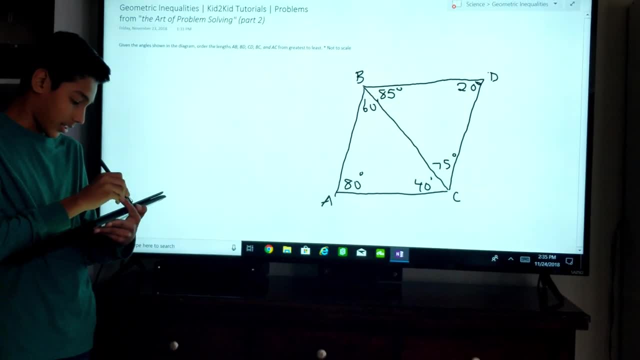 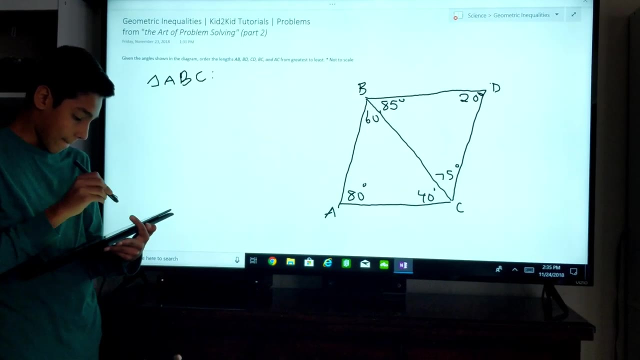 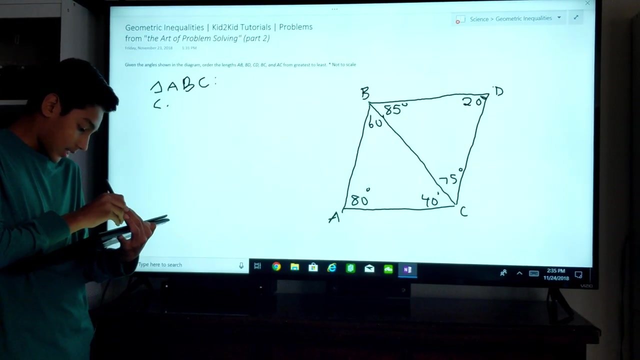 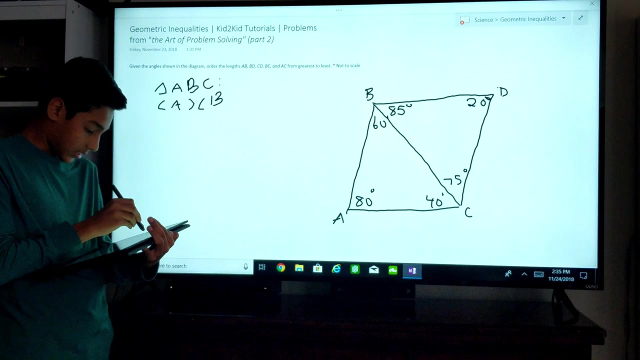 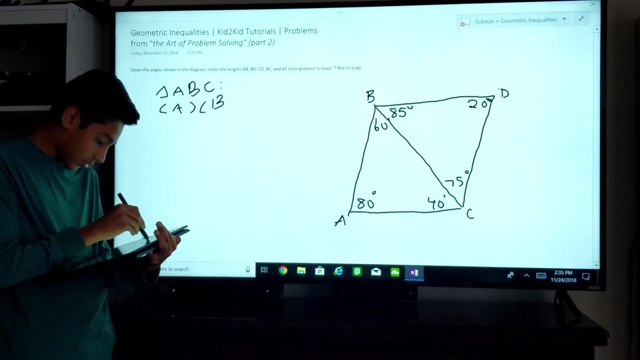 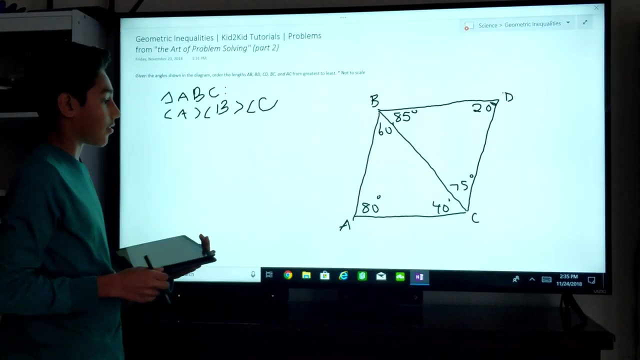 so let's focus on only triangle a b c. so triangle triangle, triangle a b c. so we know that in triangle abc, angle a is greater than angle b, which is greater than which is greater than angle C. So remember, we're only talking about triangle ABC, So this only. 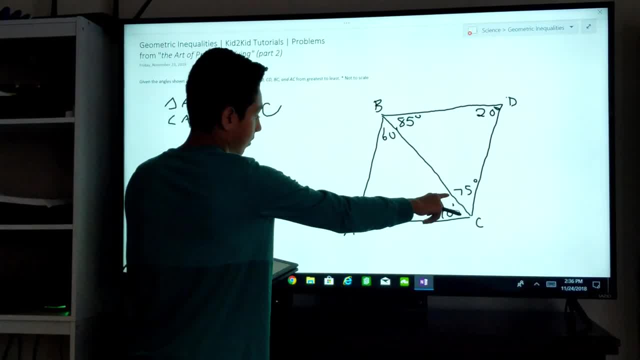 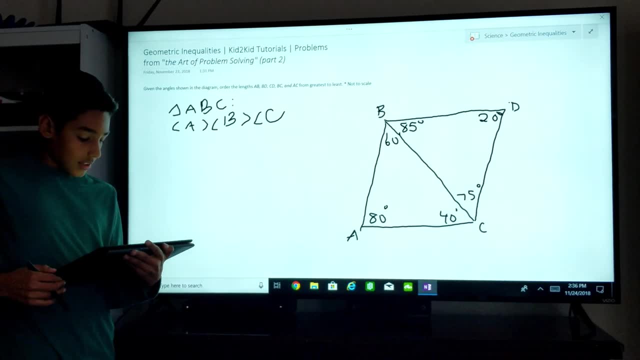 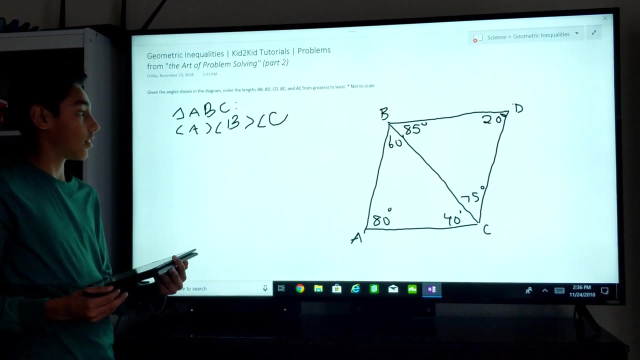 that part would be angle B, that part would be angle A and only that part would be angle C, since we're just focusing on triangle ABC. So you need to know that the measure of the angles corresponds to the length of the sides that are opposite from it. For example, since 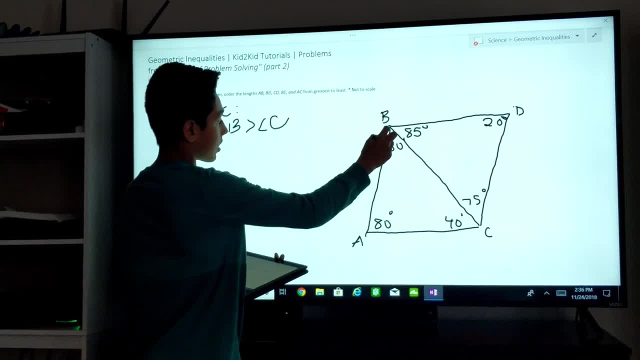 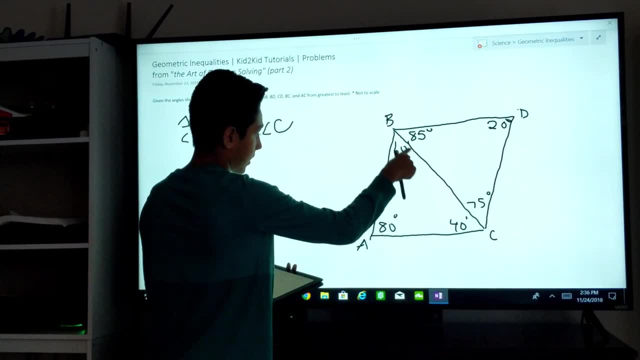 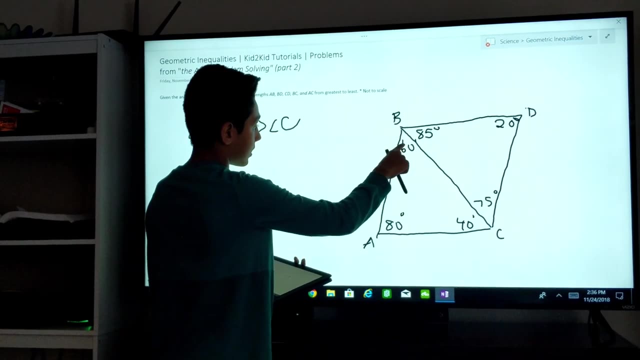 angle A is 80 degrees, which is larger than 60 degrees. this side opposite from angle A, which is BC, that's, opposite from angle A, is greater than the length of the side opposite from angle B, since angle A is greater than angle B. So AC would be less than BC. 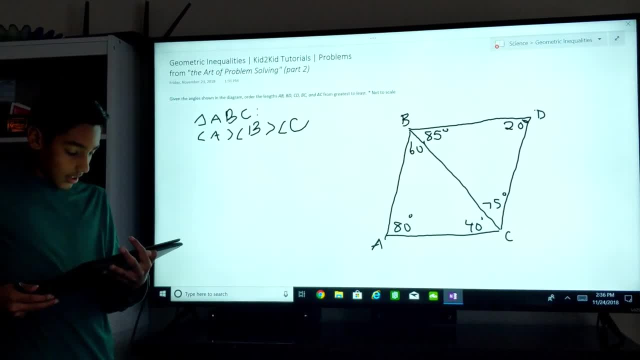 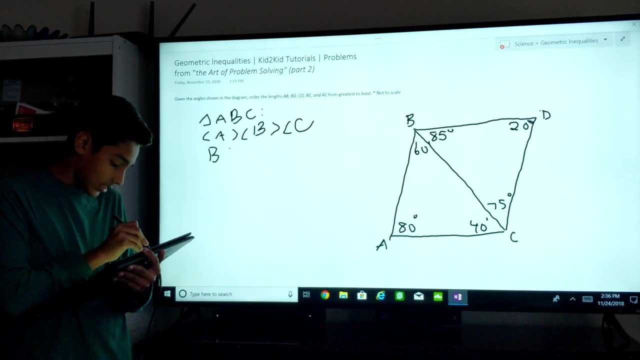 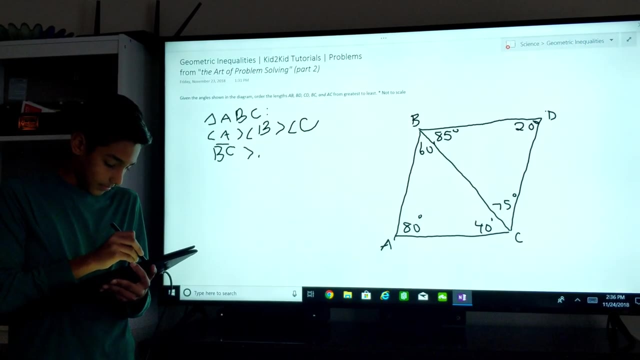 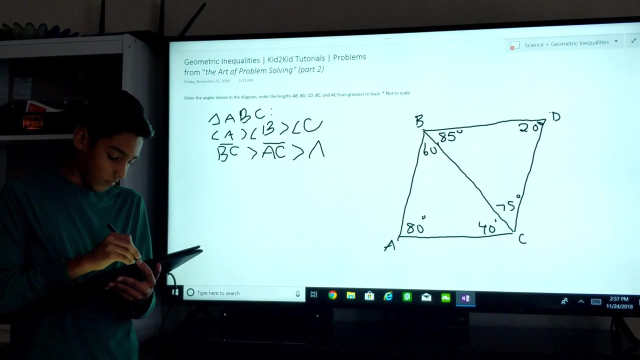 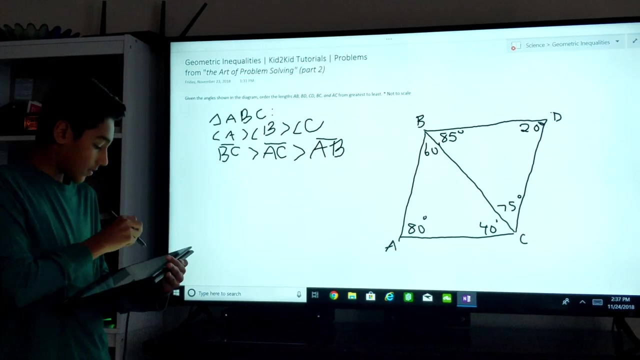 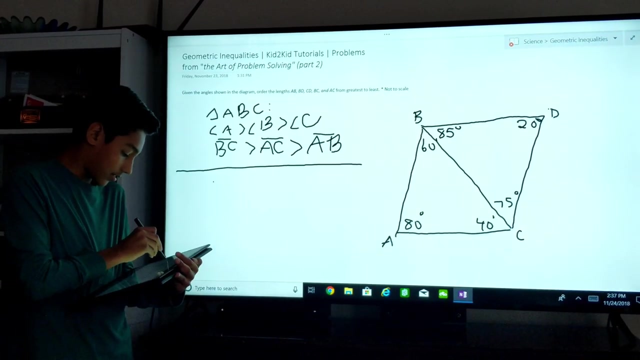 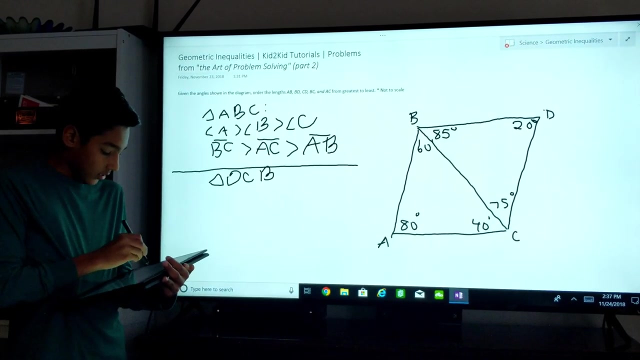 So we know that angle A is greater than angle B, so BC is greater than AC, which is greater than AB. So that's all for triangle ABC, Thank you. Now let's go over to triangle DBC or DCB. Let's go to triangle DCB. Okay, So we know. 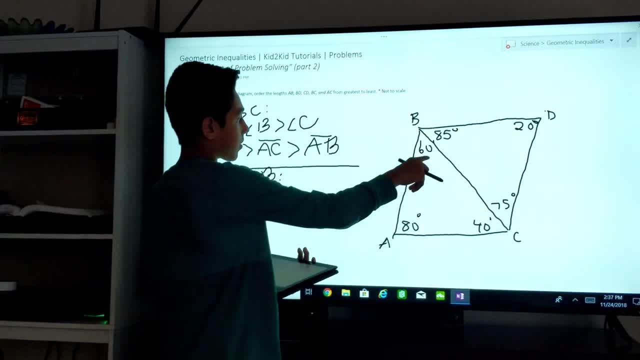 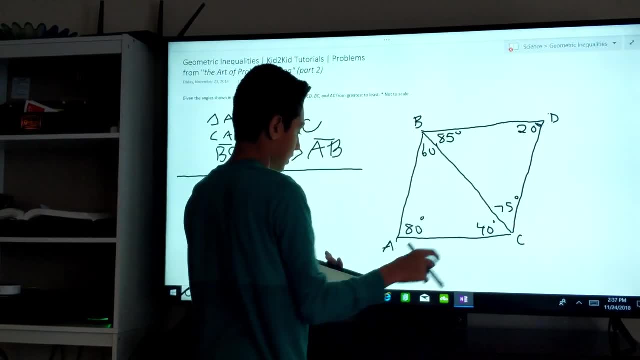 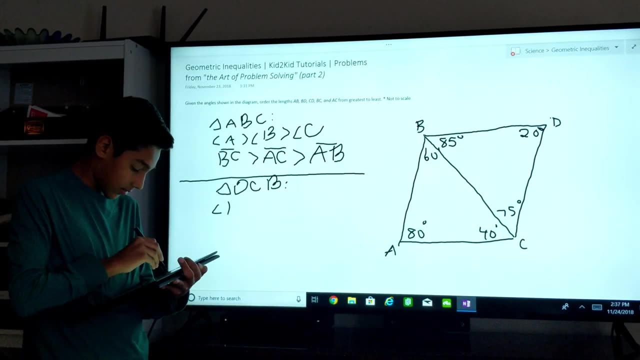 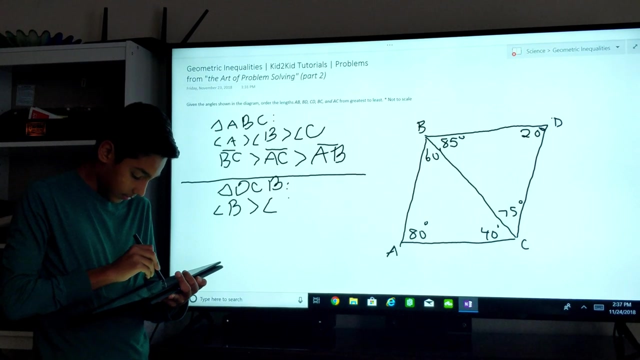 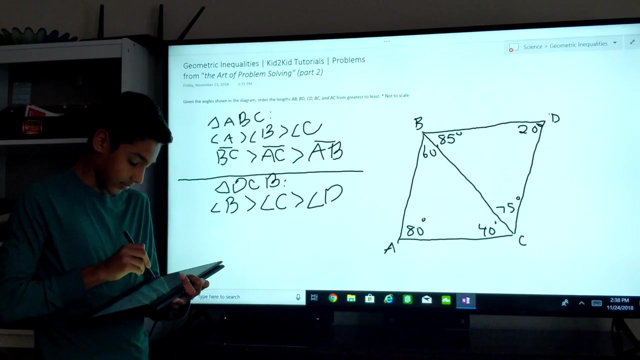 that angle B. so remember, since we're focusing on triangle DCB, only that would be angle B and only that would be angle C. So angle B is greater than angle C, which is greater than angle D. So again, like we, 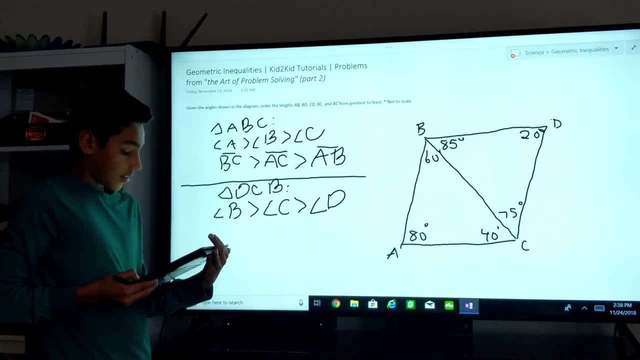 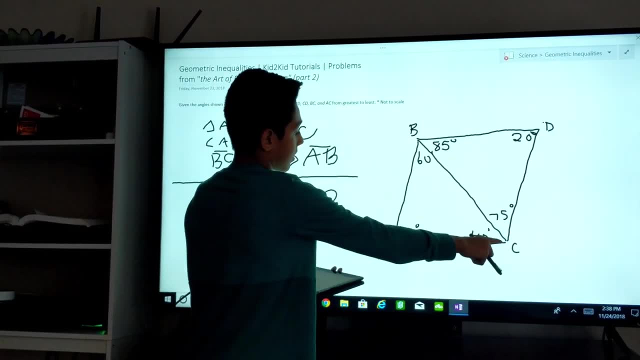 did before with triangle ABC, we know that the length of the sides correspond to the measure of the angle. So angle B is greater than angle C, which is greater than angle A. So since angle B is greater than angle C, the side opposite from angle B, which is 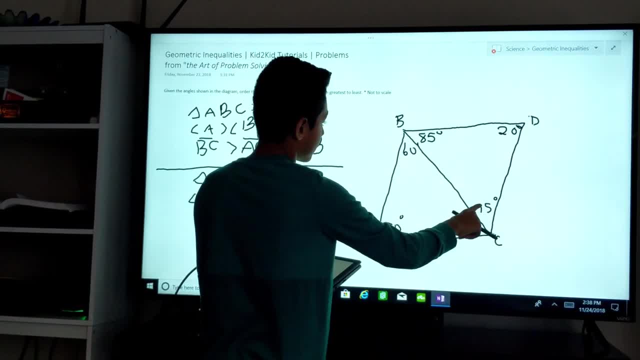 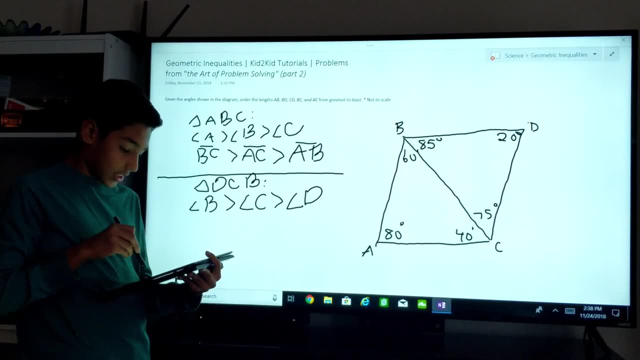 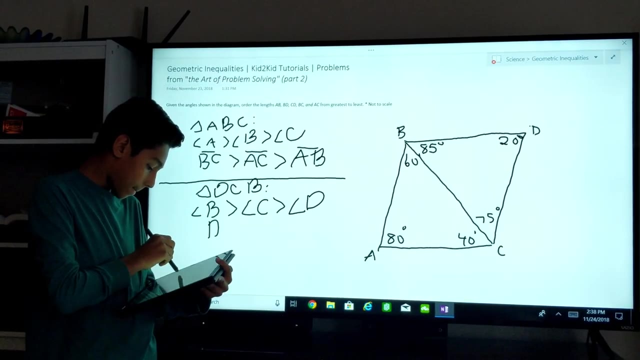 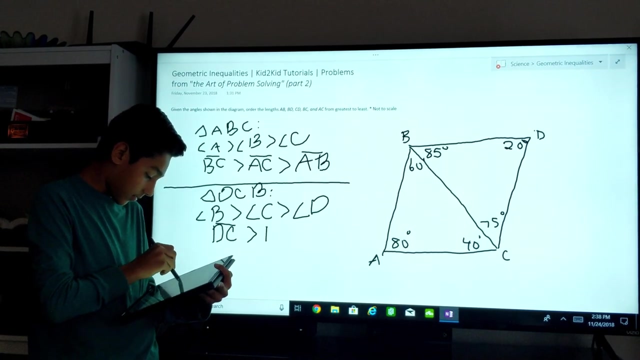 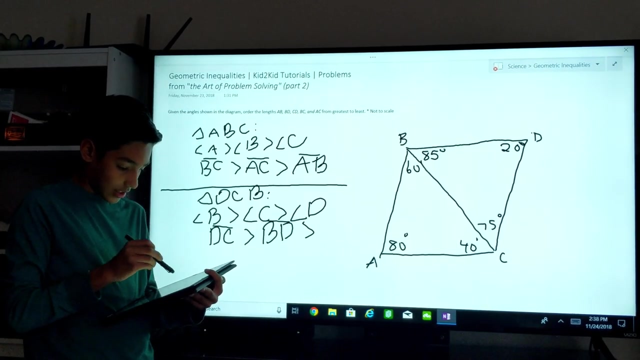 DC would be greater than the side opposite from angle C, which is BD. So angle DC, not angle DC. side DC is greater than angle BC. Okay, Okay, Okay, Okay, Okay. side BD, which is greater than. so DC is greater than BD, which is greater than BC. 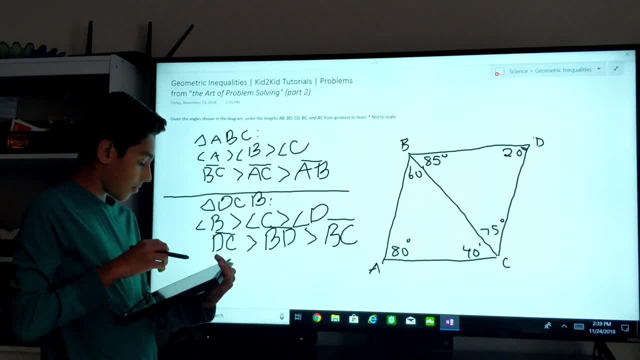 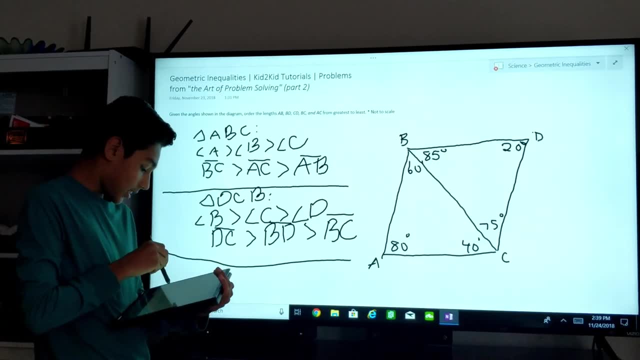 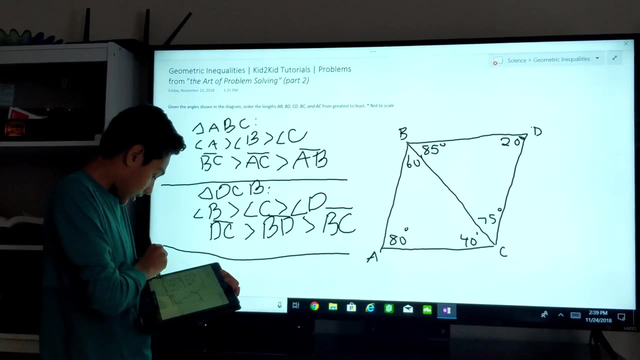 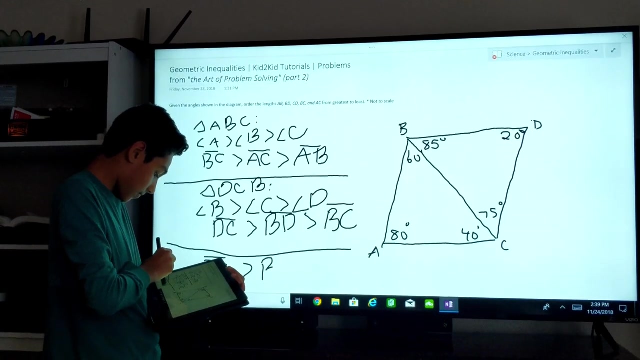 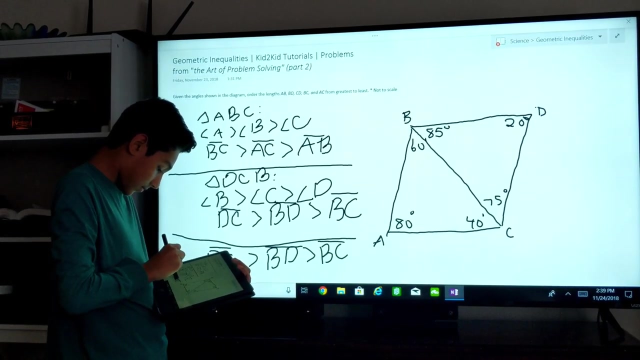 So now, since we have both of these, we can order them from order the links. So we got pretty lucky here, since BC is the least on that side but the greatest on that side on that triangle. So that means we can just do: DC is greater than greater than BD, which is greater than BC, which is greater than AC. 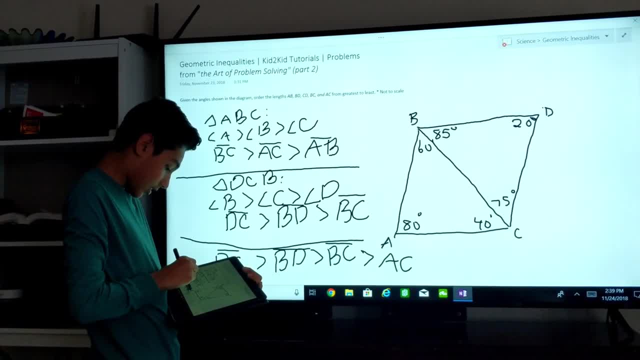 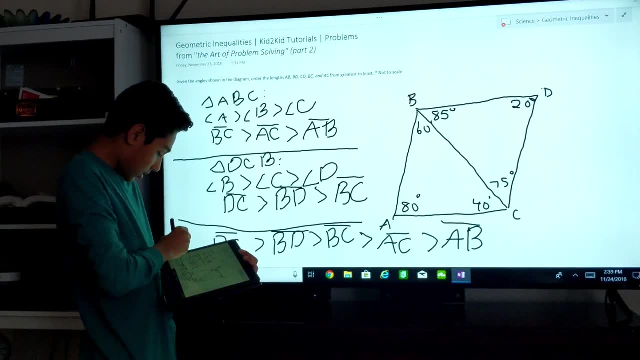 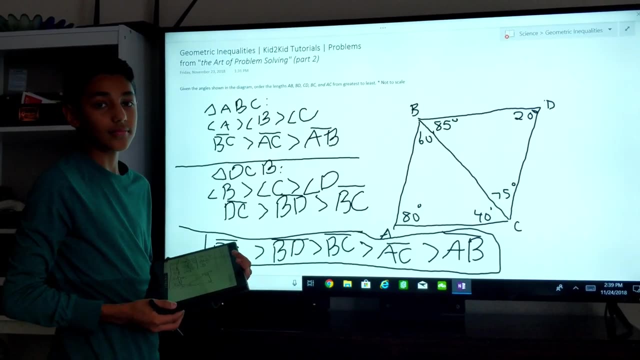 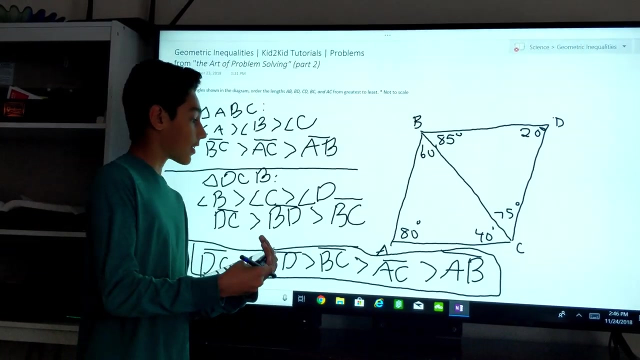 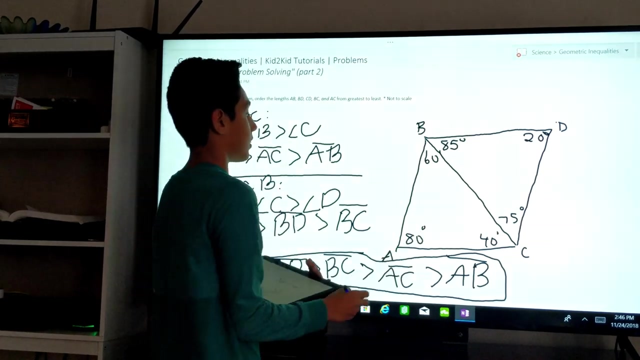 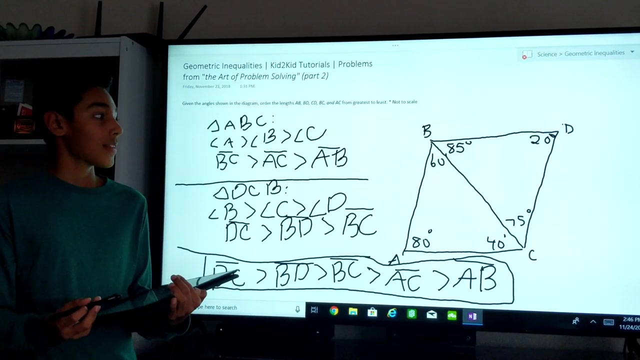 which is greater than BC And AC is greater than AB. So here is our answer. So remember when I said: like the length, the measure of the angle corresponds to the length of the side opposite from it. So you'll learn how to prove that in trigonometry, using, like, the law of sines or the law of cosines. 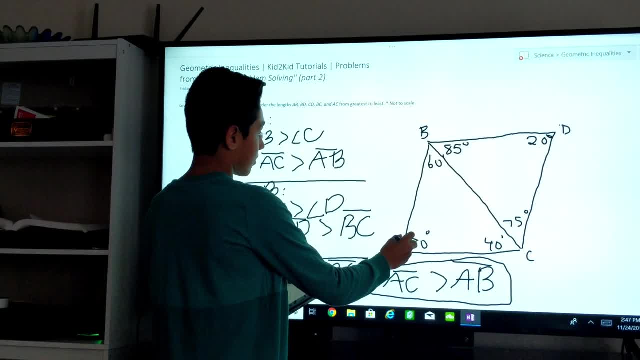 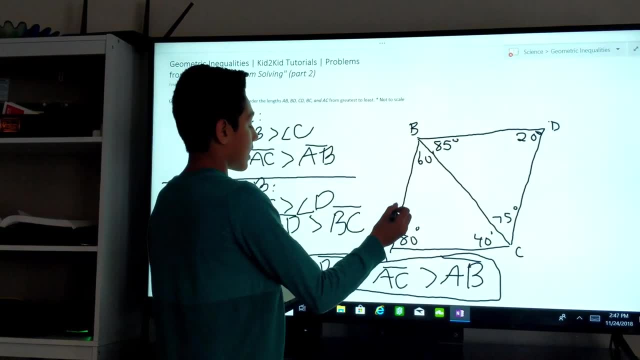 So for now, just know that the greatest angle. so find the greatest angle, the side opposite from that is the greatest side, or the longest side, And then find the second greatest angle, and then the side opposite from that is the second greatest side. 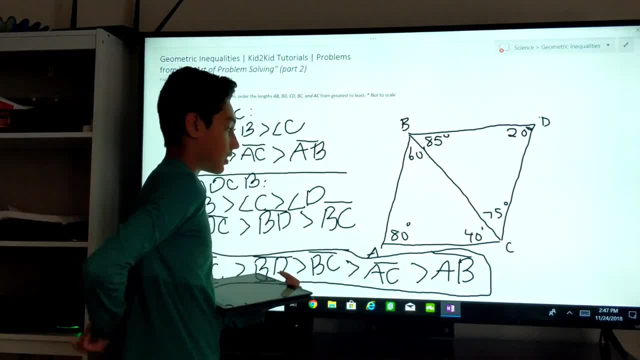 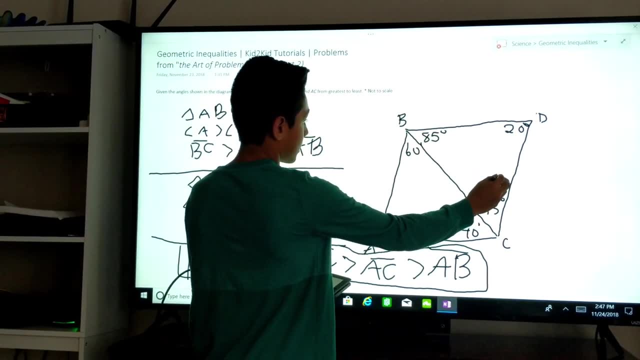 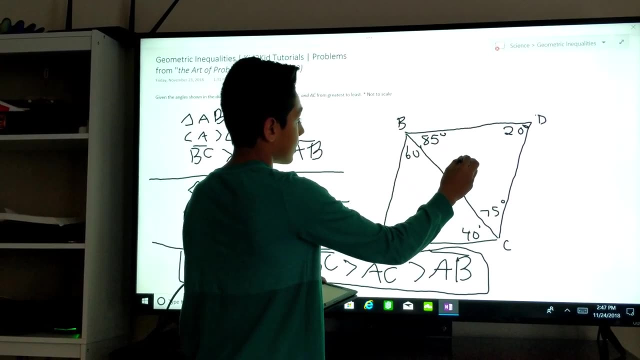 And find the smallest angle and the side opposite from that is the smallest side. So again, Okay. So again, the greatest angle, the side opposite from that is the greatest side. the second greatest angle, the side opposite from that is the second longest side. and then the smallest angle, the side opposite from that is the smallest side. 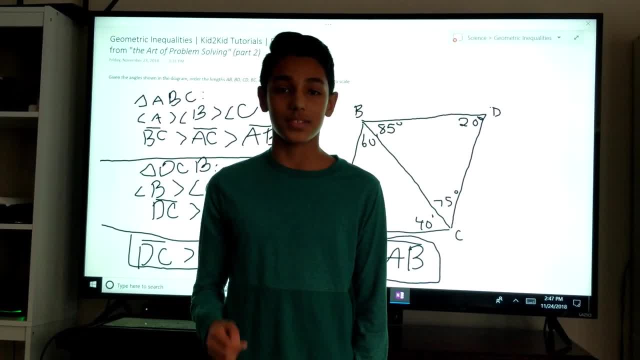 Thank you for watching Kid2Kid Tutorials and if you like our videos, please share, like and subscribe.